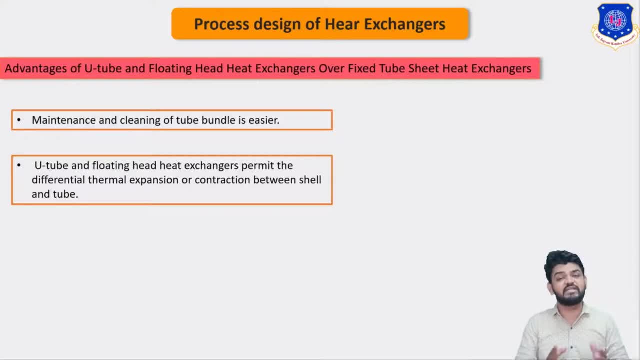 one right. So the maintenance and cleaning of such heat exchangers are very easy. But with the fixed type, or we can say fixed head tube heat exchangers, the maintenance and cleaning is rather, very difficult. right, Because we have to dismantle. 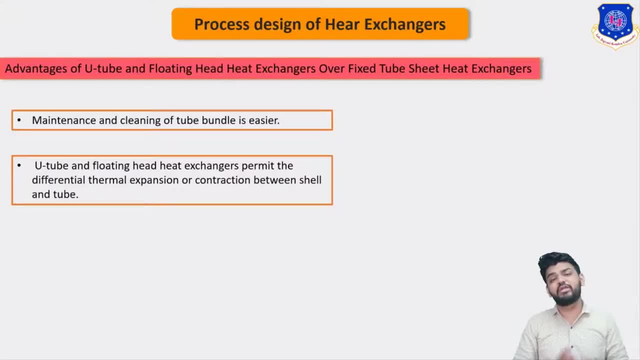 the entire heat exchanger in order to remove the tube bundle. Now the second advantage of the U-tube type or the floating head type heat exchanger is the U-tube and floating head heat exchanger permit the difference, or we can say the differential. 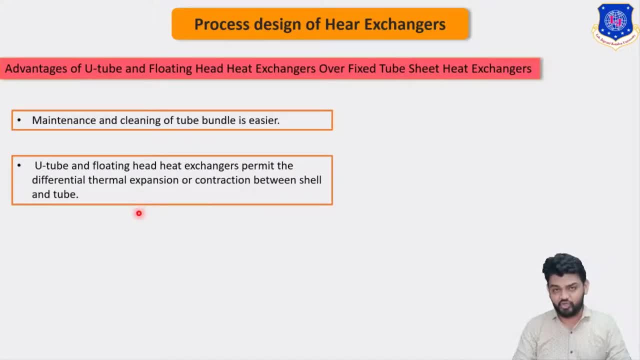 thermal expansion or the contraction between shell and tube cell. Since we are using a tube type, or we can say we are using a floating head type of the heat exchanger, they are allowing us, or they are permitting us, the thermal expansion, or we can say thermal contraction of the entire metal, Because we are using hot and cold fluid. 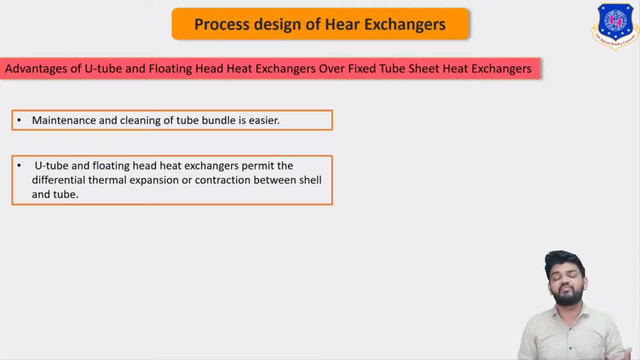 at the same time it is very obvious that we will face some kind of expansion and the contraction inside the heat exchanger so that you tube type and the floating head heat exchanger can suffice. heat exchanger provides this contraction and expansion of the matter between shell and 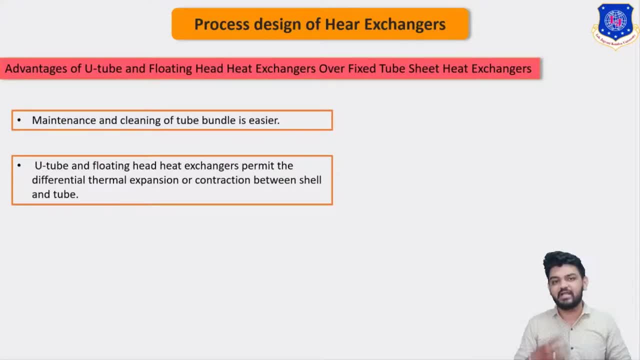 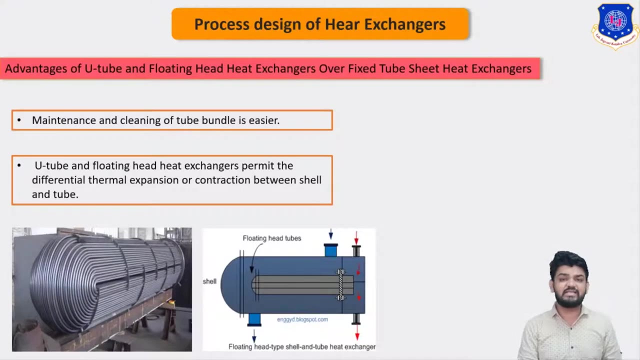 cubes. This is same case is not possible with the help of fixed tube heat exchangers. Generally, there is not enough space between shell and tube to fallacilate the expansion, or we can say contraction, of the matter, As you can see here on the image that this is the example. 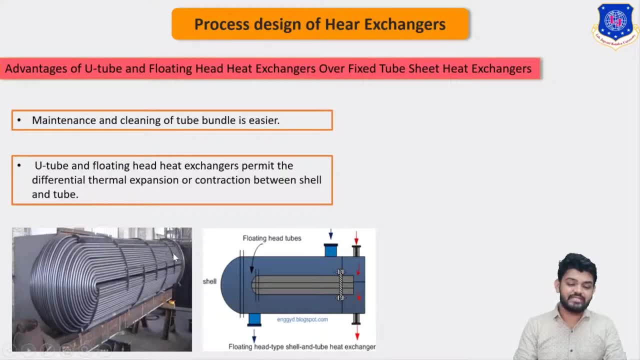 of the U-tube type heat exchanger. As you can see here, these tubes are arranged in a U-type shape, So this is why this type of heat exchanger is called as U-tube shell and tube heat exchanger, While this is the floating head type of the heat exchanger, in which the 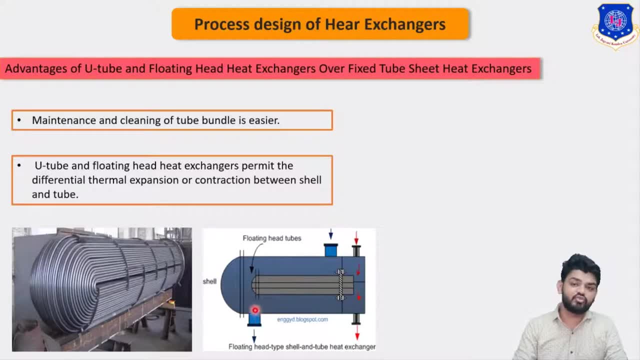 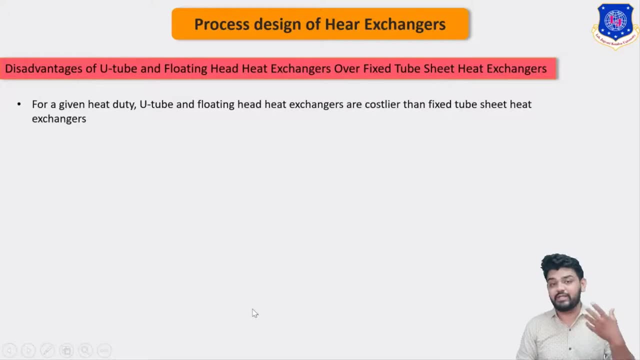 head of tube bundle is being allowed to float inside the shell. Now if we discuss about the disadvantages of U-tube and floating head type of the heat exchanger, then we can say that for a given duty, U-tube and the floating head type heat exchanger are costlier than 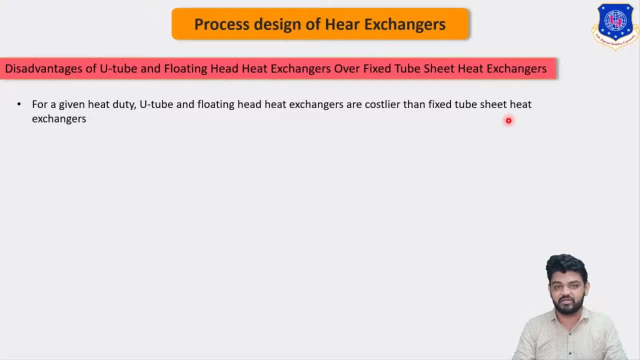 the tube than the fixed tube type of the heat exchanger. So this U-tube and floating head type of heat exchanger are generally very much costly than the fixed type of the tube heat exchanger. Well, you can easily understand that it is not that much easy to make U-shape. 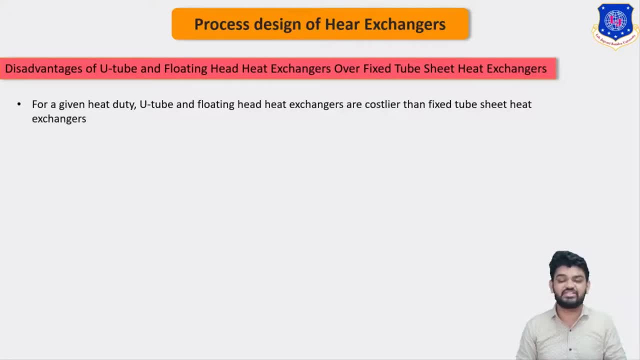 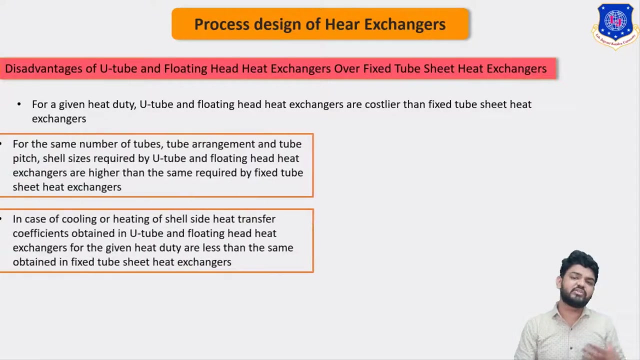 out of the tube. So this is why this type of the heat exchanger are rather, very costly than the fixed type of the tube heat exchanger. There are many reasons behind the cost difference of U-tube and the floating head. Here the two main reasons are explained. you can see here that for same 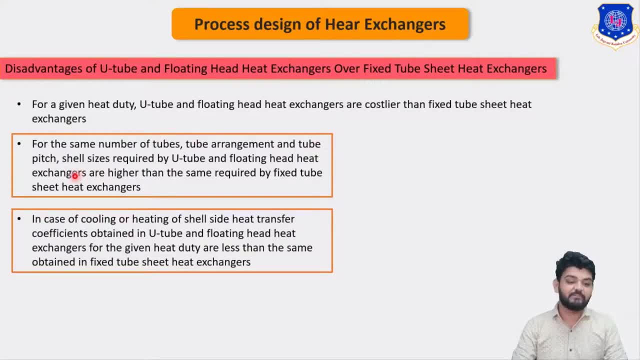 number of tube, the tube arrangement and tube pitch shells as required by U-tube and the floating head, is much greater than the fixed type of the tube heat exchanger. So this is why this type of the heat exchanger are rather very costly than the fixed type of the tube. 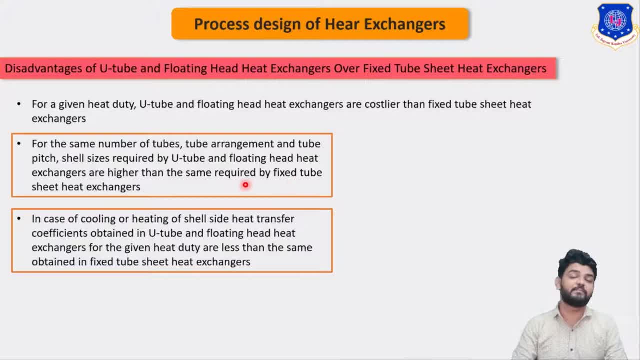 heat exchanger. So the cost of the heat exchanger is greater than the size required by the fixed tube sheet or we can say fixed tube heat exchanger. So with the case of U-tube type shell and tube heat exchanger and the floating head type shell and tube heat exchanger, the shell diameter 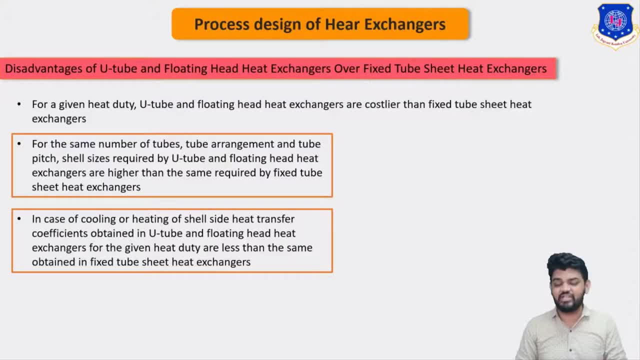 required is very large and we have already understand in the previous lecture. the cost of heat exchanger is greaterly depends on the diameter of the shell. So if we require greater diameter of shell In the case of U-tube and floating head, ultimately it will increase the capital cost of heat exchanger. 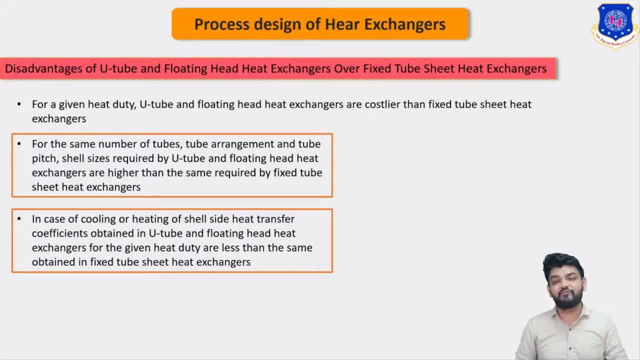 right, but on the opposite side, with the help of fixed type of the tube heat exchanger, the cost of- or we can say the diameter of shell is very much less. So this is the main reason that's why the cost of U-tube or the floating head heat exchanger is much more than the 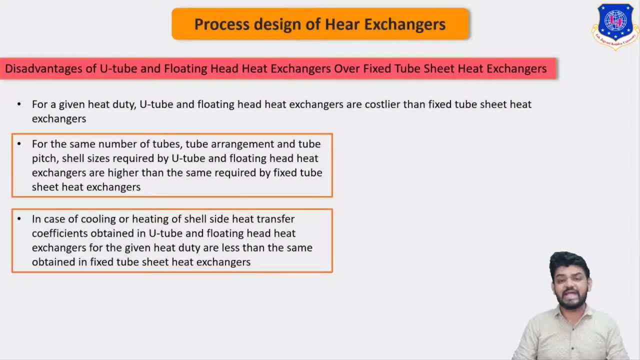 cost of fixed tube heat exchangers. Now the second point is like in the case of U-tube or the floating head heat exchanger. In case of cooling or heating shell and heat transfer coefficient obtained in U-tube or the floating head heat exchanger is very much less than. 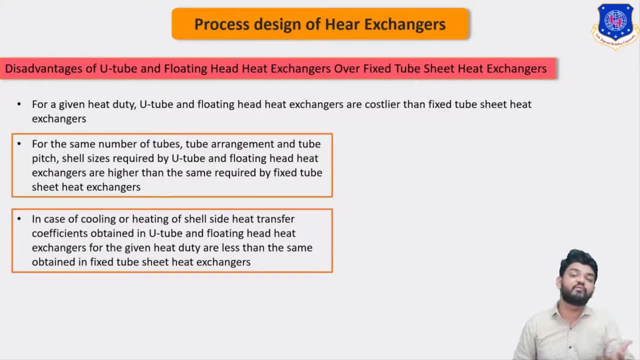 the heat transfer coefficient obtained from the fixed tube type of the heat exchanger. So the U-tube and floating head gives lesser heat transfer coefficient and the fixed tube type of the heat exchanger gives higher amount of the heat transfer coefficient. So these are the main disadvantages. 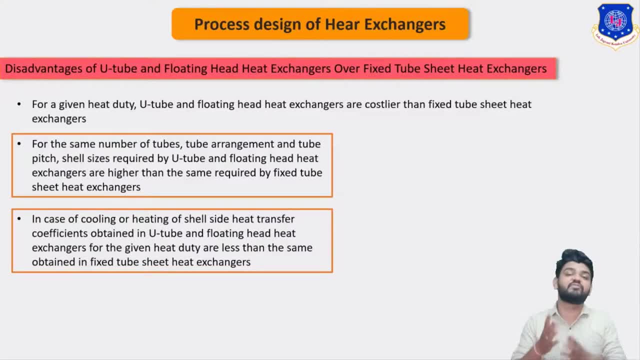 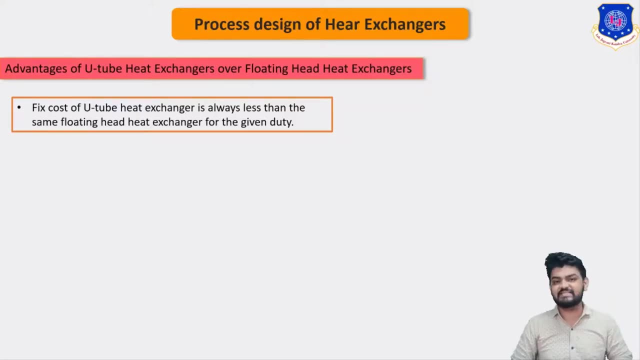 advantages of the U tube, or we can say floating head type of the heat exchangers versus the fixed tube type of the heat exchangers right Now. next, we are going to understand the advantages and disadvantages of U tube heat exchangers versus floating head type of the heat exchanger right. 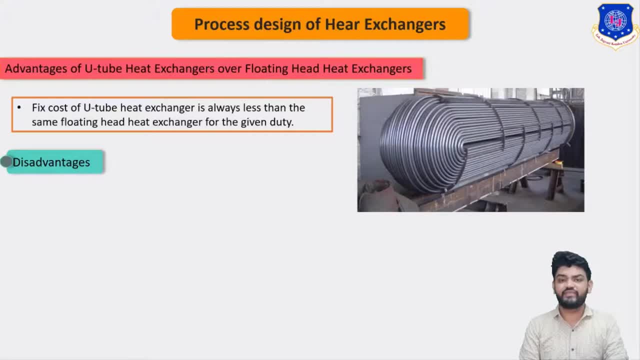 So, as you can see here, these are the advantages of the U tube heat exchanger. As you can see here, fixed cost of U tube heat exchanger is always less than the floating head of the heat exchanger right. So this is the only advantage of the U tube heat exchanger: that it cost will be lesser. 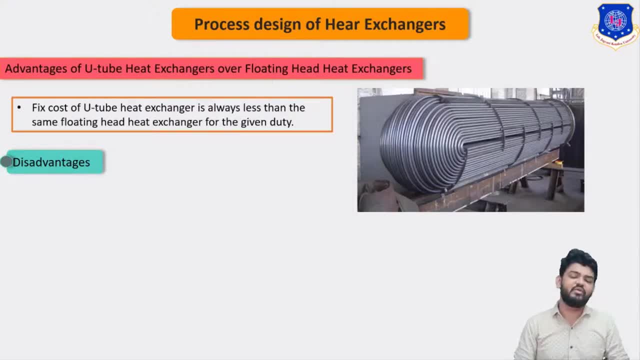 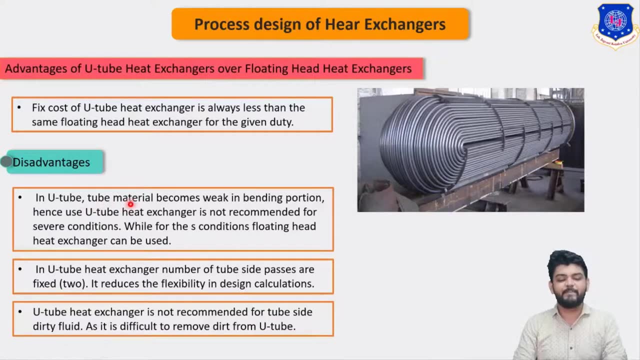 than the floating head type of the heat exchanger. right Now, if we look at the disadvantages of U tube heat exchanger then we have in the U tube tube material become weak in the band proportion right With the U tube type heat exchanger. 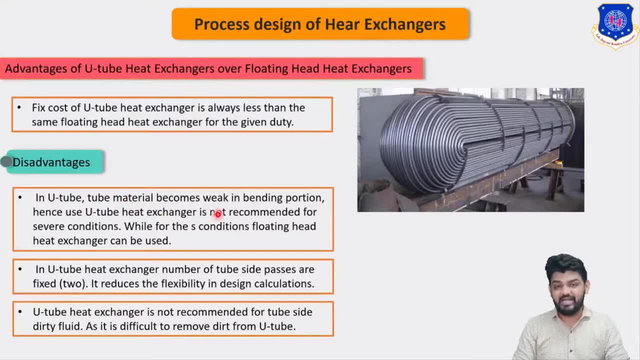 The tubes become weak at the banding position, right? So, as you can see here, in this particular position, or we can say, at this particular portion of the heat exchanger, our tubes become weak since we are banding it, So it will lose its strength, right? 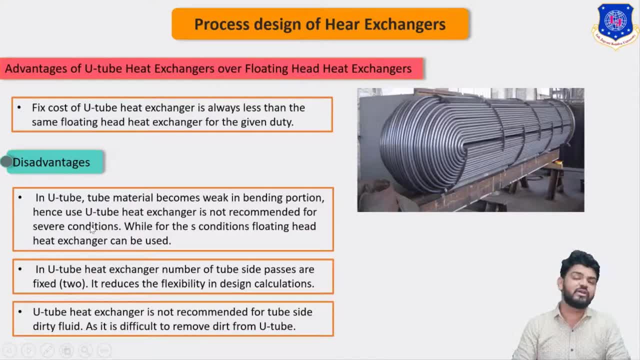 So hence, use of heat exchanger is not recommended for different conditions where we have to encounter very high velocity or, we can say, very high volumetric flow rate, right? So, while for the same condition, The floating head heat exchanger can be used because it do not involve any banding of the 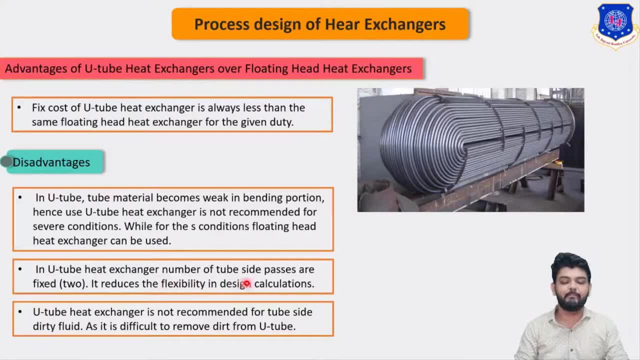 tubes right. Now in the U tube heat exchanger the number of tube passes are fixed. that is tube right. So with the case of U tube type of the heat exchanger we can only achieve two times passes for the tube side material right. But this ultimately reduce the flexibility and process designing of the U tube type of. 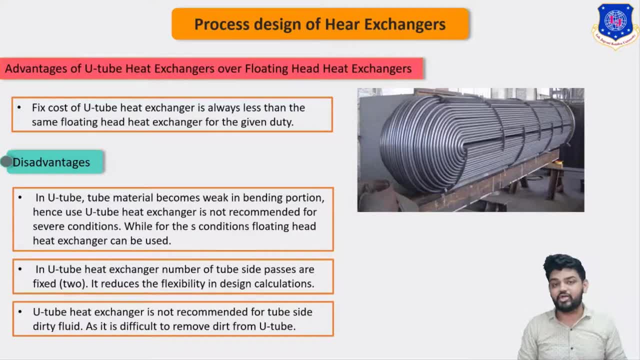 the heat exchanger right. So we have seen that In order to achieve this, In order to increase the heat transfer coefficient for the tube side, we have to select multiple passes for the tube side material right. and then the last disadvantage of U tube is that 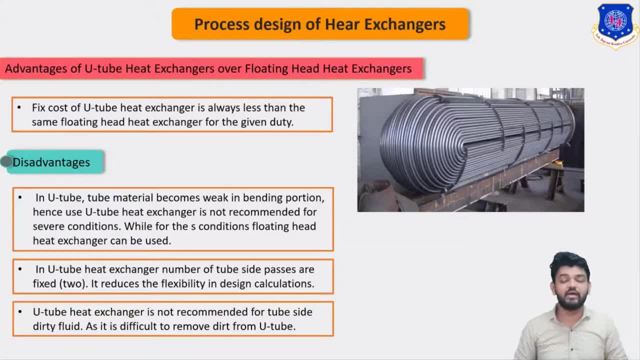 U tube type of the heat exchangers are not recommended when the tube side fluid is very dirty, right, because it will ultimately chop, or we can say block, the U shape in the tubes, right. So these are all the disadvantage of the U tube heat exchangers against the tube side. 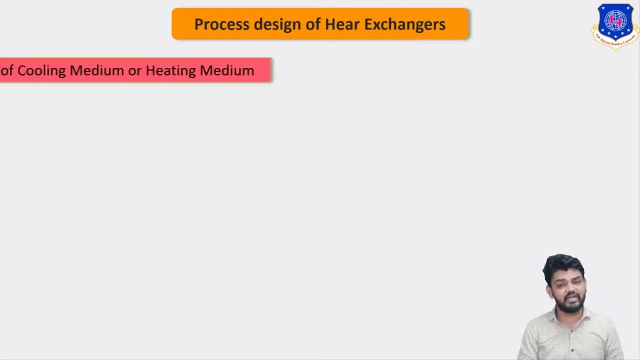 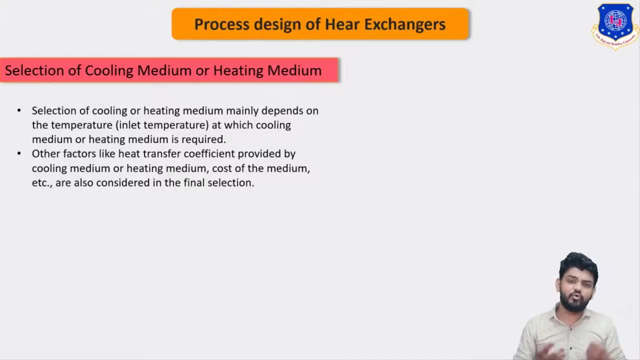 material right. So the next thing is the selection of cooling and heating medium. Well, the selection of cooling and heating medium is again very crucial parameter for the designing of heat exchanger. As you can see here, the selection of the heating and cooling medium will greatly depend on. 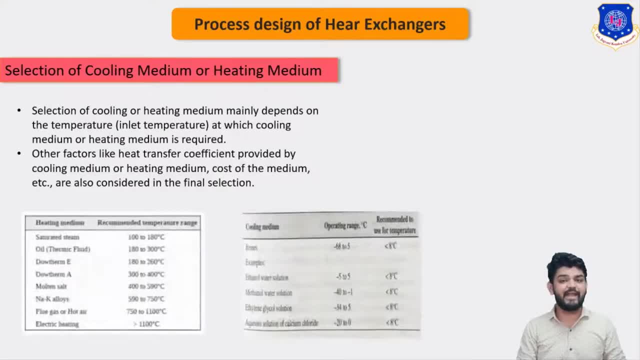 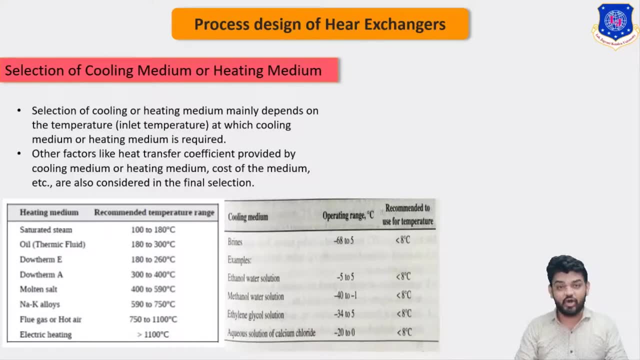 the inlet temperature at which we want to provide cooling and heating right. So other factor are also be considered, while seeing that the kuinly temperature is not sufficient, So the temperature is not sufficient, So the temperature is not sufficient right selecting the heating and cooling medium. these factors are: heat transfer coefficient provided. 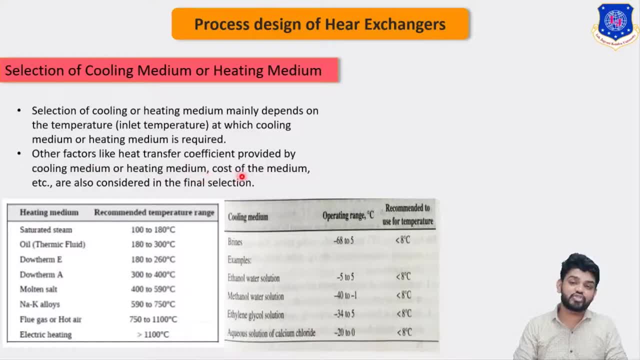 by cooling medium or the heating medium, then the cost of the cooling or heating medium: right. so these are all the heating medium that are available for the heating purpose and these are the all cooling medium if we want to achieve some temperature around 300 to 400 degree Celsius, and we need to use this down thumb key, right if we want to have higher. 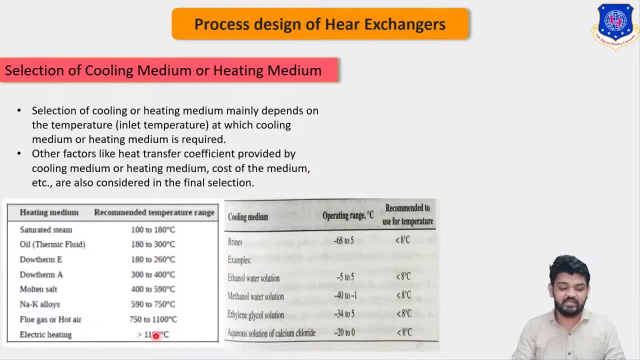 temperature than the 1100 degree Celsius, then we have to use electrical heating right and again, as you can see here that this standard saturated steam can be used to achieve temperature of 100 to 180 degree Celsius, while in the case of cooling medium, if we want to cool, 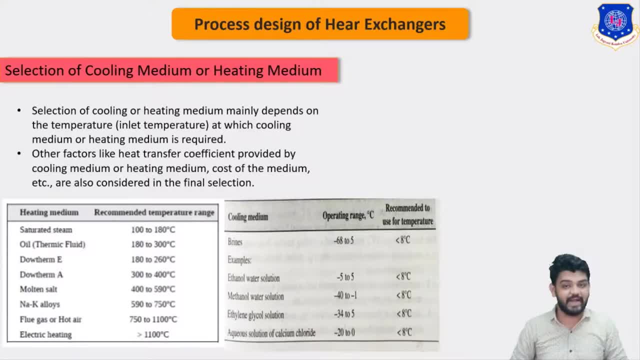 one material up to 8 degree Celsius, then we can use bright. or if we want to achieve higher cooling, up to minus 20 degree Celsius, then we can use electrical heating, right, and again this ethylene glycol solution, right. so these are all the cooling medium and heating medium. 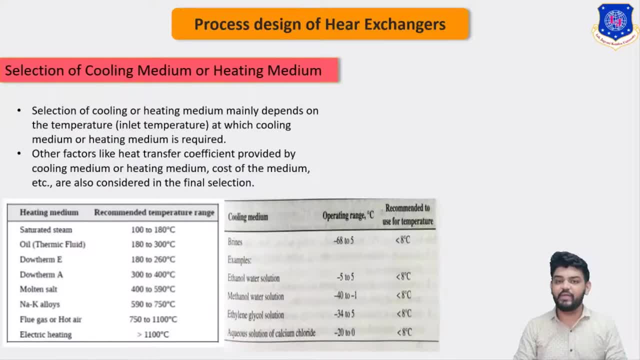 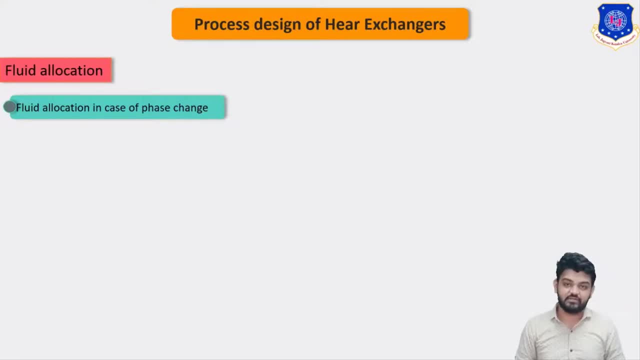 that are being used in a industrial level right now. if we move to the next topic in the designing of shell and tube heat exchanger, then it is the fluid allocation, right? so this point is again very important for the GTU exam, right? as you can see here: fluid allocation. 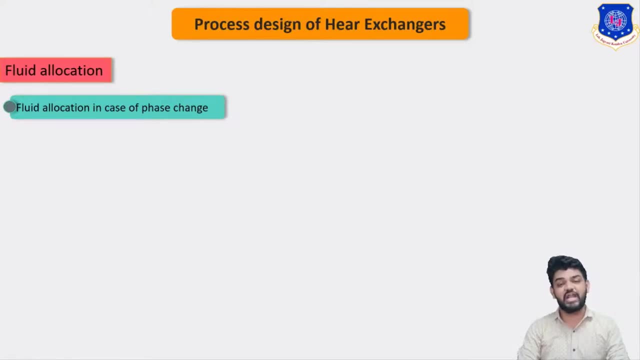 is very important part of the designing of shell and tube heat exchanger. so let us understand the fluid allocation in the case of phase change. so whenever there is a phase change occurring while transferring heat from one fluid to another fluid, we need to consider these parameters. as you can see here, condensing or the vaporizing fluid is normally taken. 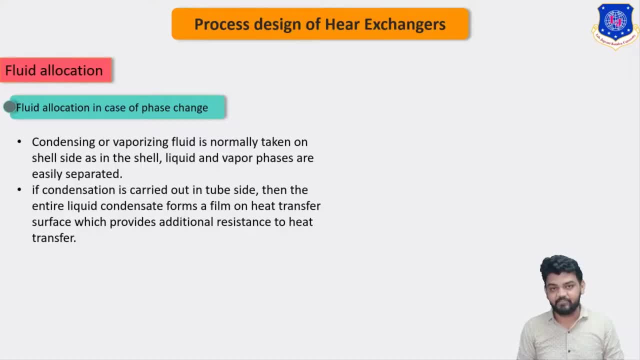 on the shell side in the shell and tube heat exchanger. so fluid which has to tendency to boil, or we can say it has to tendency to condense during the heat transfer, that fluid is need to be fastened. This is being only done because we can easily separate liquid and vapor that is being formed. 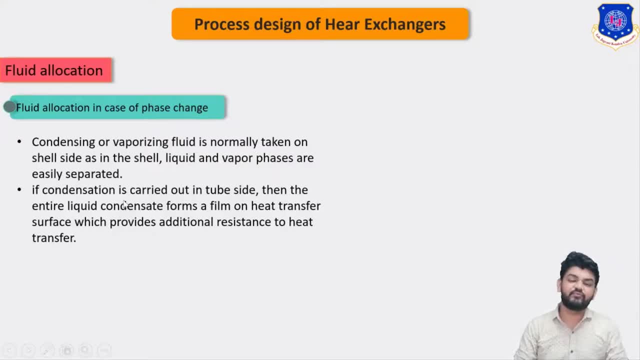 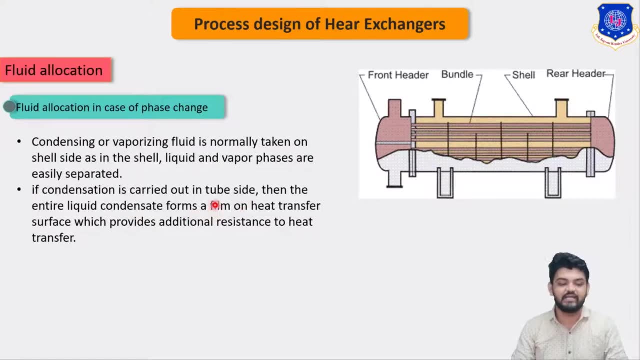 while transferring the heat right. and again, if and as you can see here in this image- if the condensation is being carried out on the tube side, then the entire liquid will condense on the surface, or we can say on the wall of tube right, and it will ultimately increase. 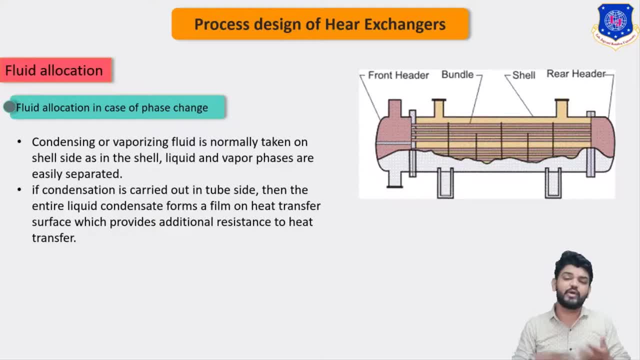 the resistance that heat has to face right. So it will ultimately increase the resistance that heat has to face right. so it will ultimately increase the thermal resistance and it will also decrease the heat transfer coefficient for the tube side. so generally the liquid, or we can say fluid, that has a tendency to 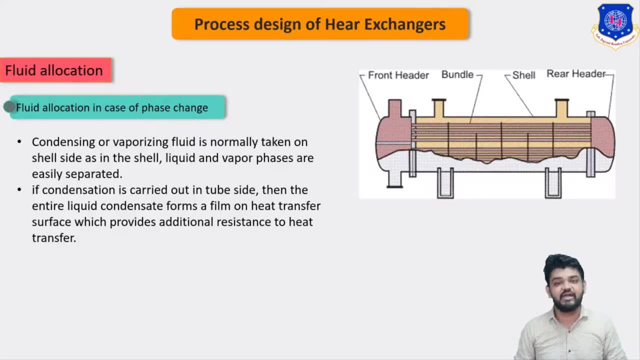 change. its phase is being palisade on the shell side, as you can see here in this image. this is the fluid that has the tendency to condense right. so when the fluid will condense, it will provide additional resistance to transfer heat in this particular area. so in the shell, 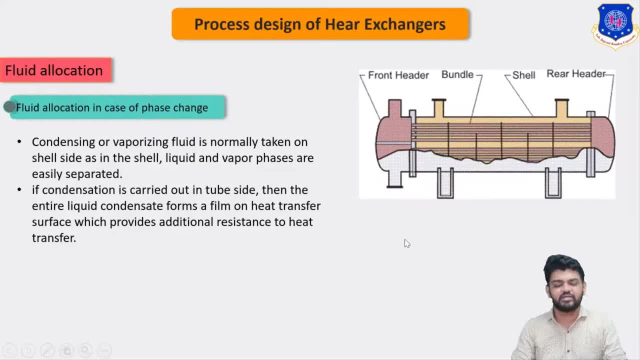 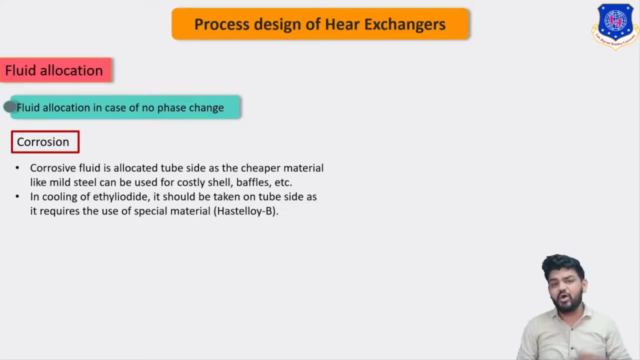 side So we can easily remove this liquid from the outlet, so fluid which has tendency to change its phase. it is always palisade on the shell side, right Now, if we look at to the fluid allocation in the case of no phase change, right so when? 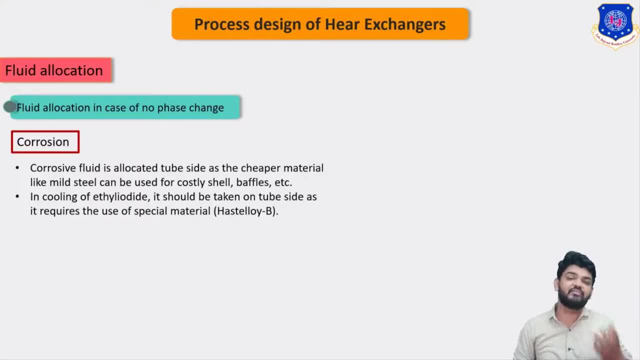 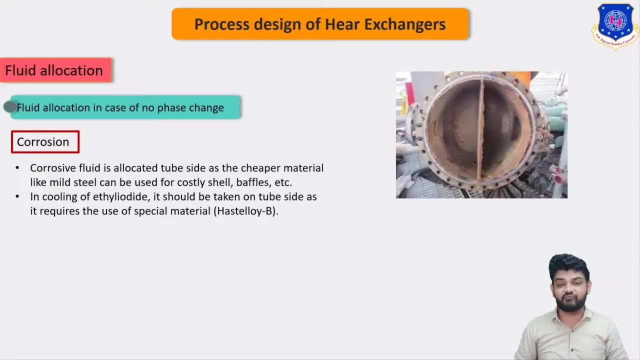 there is no phase change during the heat transfer process, then we need to consider multiple options. right, then we have to consider different parameters. the first parameter is, of course, the corrosion, So generally The fluid which has much more tendency to corrode the matter, it being palisade on the. 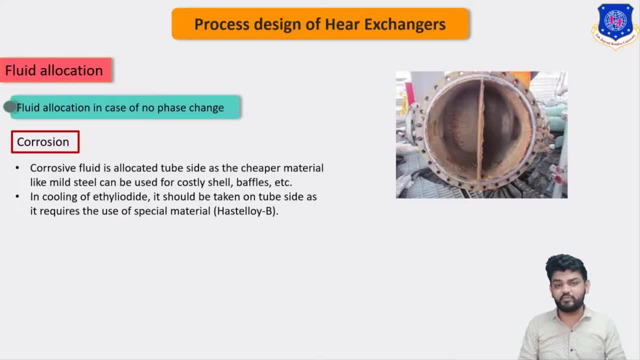 tube side, because the material used for the tube side can easily be reconstructed or it is generally cheaper than the shell side, right. so, as you can see here, corrosive fluid are allocated on the tube side, as the cheaper material is, such as mild steel, can be used. 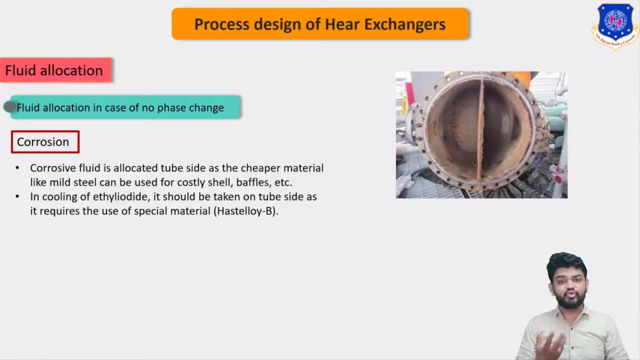 for the construction of the tubes right, if we use known corrosive metal for the construction of the cell side, that it will ultimately increase the capital cost of heat exchangers. So generally the material which has corrosiveness, tendency to corrosive metal, it being used on 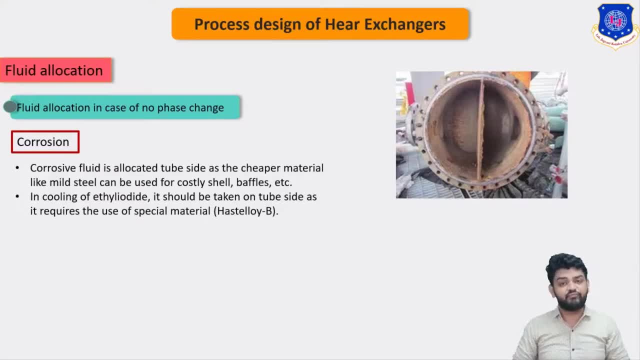 the. so generally the fluid which has tendency to corrode metal is being palisade on the tube side right. you can see here one example: in the cooling of ethyl iodine it should taken on the tube side right Because it requires special material to construct the tubes. so if we use this special material, 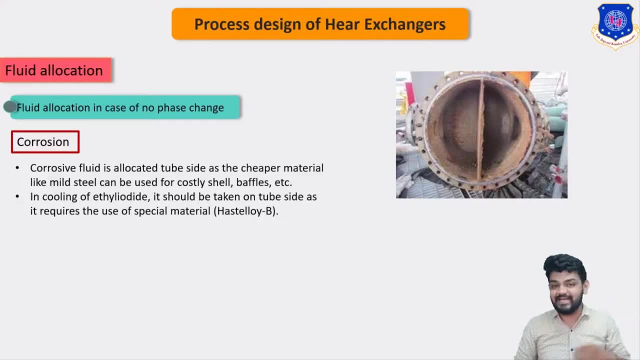 in order to construct entire shell, then it will ultimately increase the cost of shell and tube heat exchangers. Now the second parameter is the fouling. again, this fouling is very important parameter while deciding the while allocating the fluid right in a fixed tube heat exchanger inside surface. 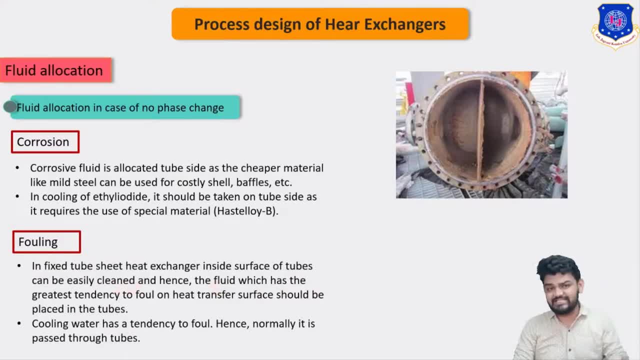 of tube So we can easily clean. right, so we can felicitate this fouling type of the fluid on the tube side. right, since we are using the u tube type or we can say floating head type heat exchanger, we can easily clear or we can say easily clean up all the fouling material over the top of 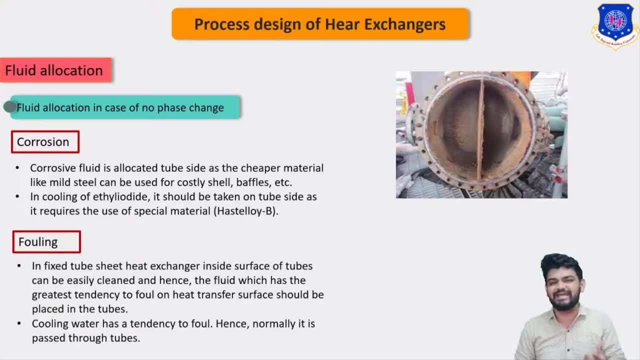 the tube side right, but the same is not possible with the case of the shell side. So generally a fluid which has tendency to foul the metal is being felicitate on the tube side right. As you can see here in the cooling water has tendency to foul on the surface of matter. 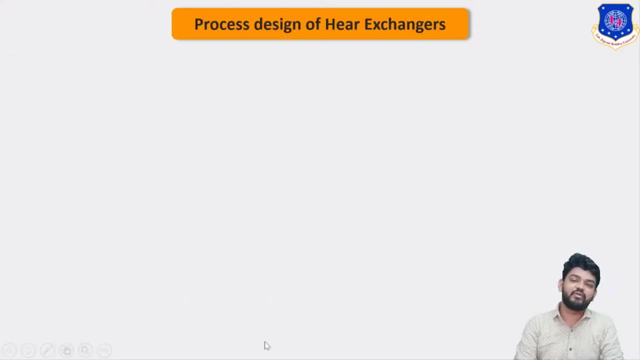 so it is normally passed through the tubes. Now if we look at to another parameter for the fluid allocation than it is fluid temperature. so at very high temperature or at very low temperature, special material is being used to construct tubes or the shells right. so such kind of materials are very costly. so 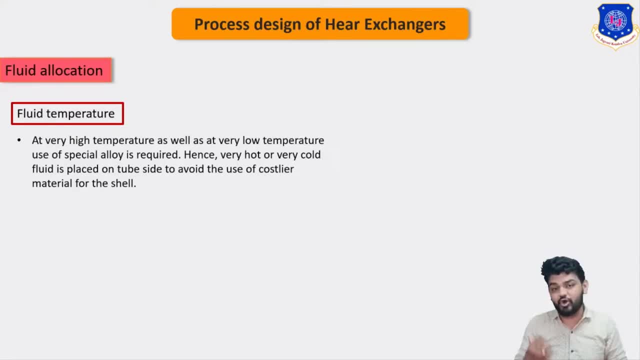 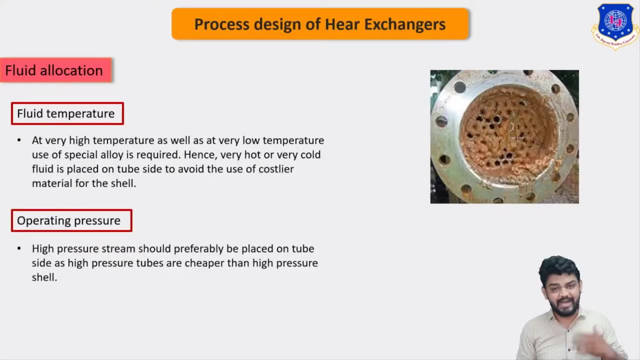 when we required very high temperature or we require very low temperature. such type of the fluids are generally being flown through the tubes right now. the next parameter is the operating pressure. so, as you can see here, high pressure stream should be preferably placed on the tube side, as high pressure tubes are. 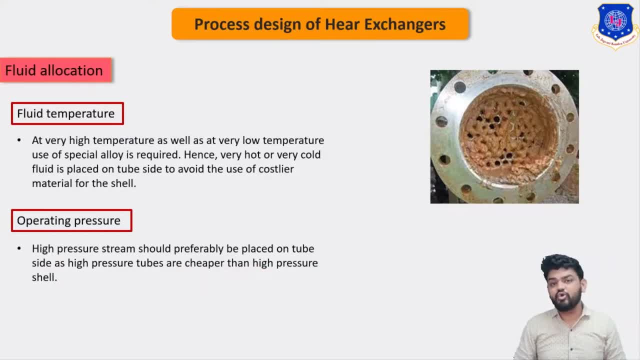 very cheaper than the high pressure cell. so to withstand the high pressure of fluid we require special type of the material right, and this special type of the material is again very costly. so to construct the tube out of the spatial material is relatively less costlier than the 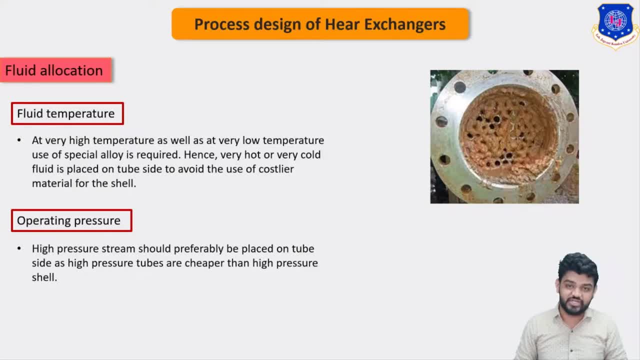 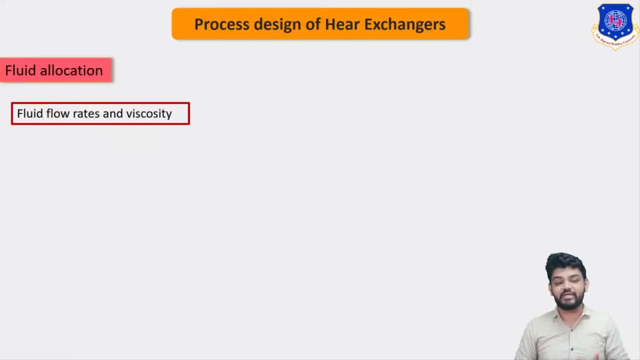 construct entire shell with the such type of the spatial material. so with the case of higher operating pressure, we are generally felicitating such fluid through the tubes right. so now let's just discuss the last parameter that need to be considered for the fluid allocation, and that 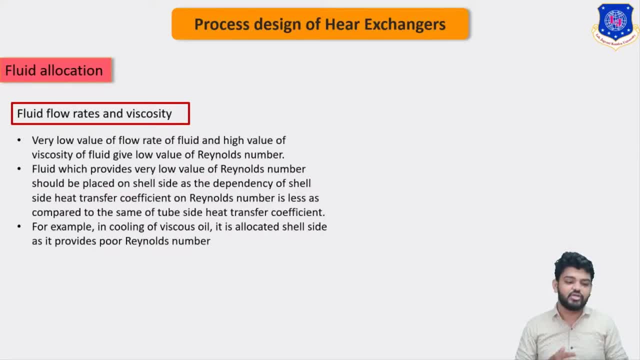 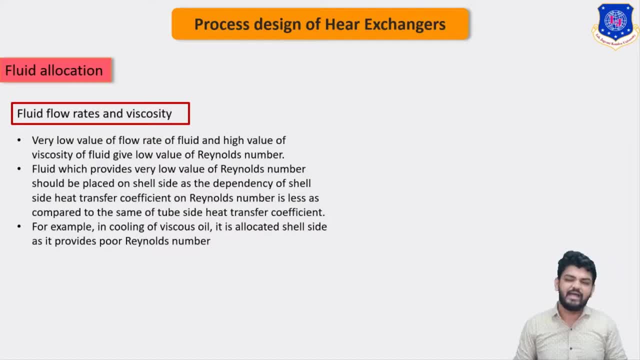 it also reduces the heat transfer coefficient and we cannot achieve the desired heat transfer through the process right. so, as you can see here, fluid which provides very low value of reynolds number. that means it has very low flow rate and it has very low flow rate and it has very low flow. 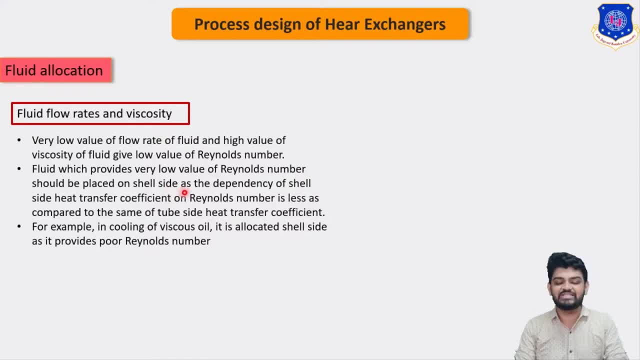 rate and very high viscosity should be placed on the shell side as its dependency of the shell side heat transfer coefficient is relatively low on the reynolds, so the fluid which has very low reynolds number are being generally used to fallixulate on the shells because the cell side heat transfer 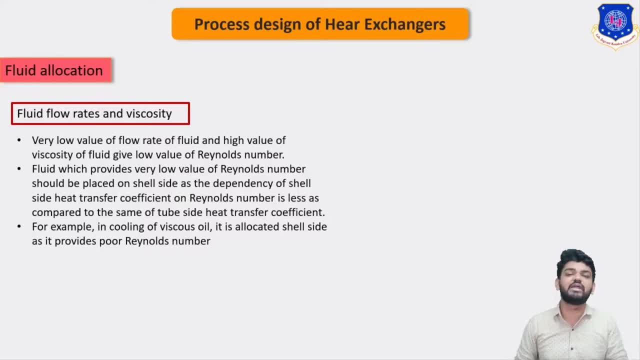 coefficient is relatively less dependent on the reynolds number, while the reynolds number is being largely affected on the heat transfer coefficient for the tube side. so we are always required or we are always providing the high a fluid which has higher reynolds number on the tube side right. so 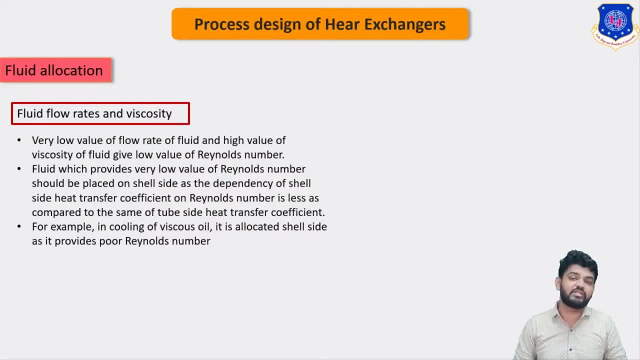 this is what all about the fluid allocation for the heat exchangers. this point is again very important, right? so let's just quickly revise it. we have understand that if the phase change type of the fluid is going to be higher than the reynolds number, then the heat transfer coefficient 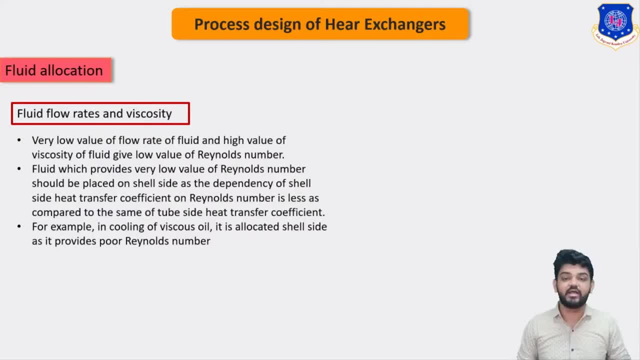 need to be allocated in the shell and tube heat exchanger, then it has to be fallixulate on the shell side right, as we can easily remove vapor and liquid from the shell side, while with the case of the fluid, which do not involve phase transfer during the heat transfer process, we need to 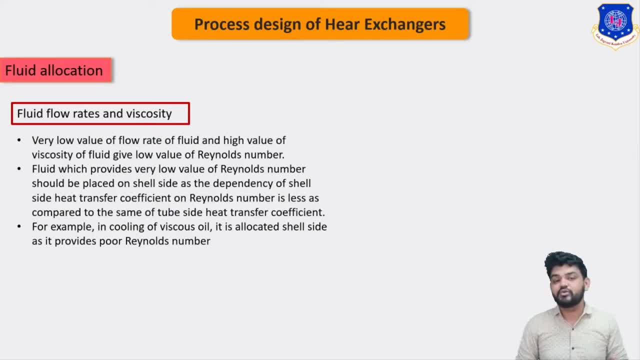 consider different parameters, such as corrosion, so corrosive fluid are always provided for the tube side, right, then we have seen fouling, so material which has tendency to fallixulate on the metal are being provided, or we can say fallixulate on the tube side. then we have seen the temperature.